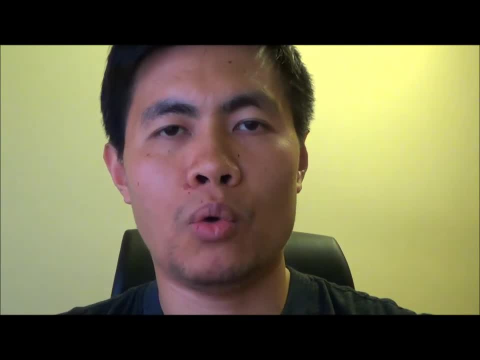 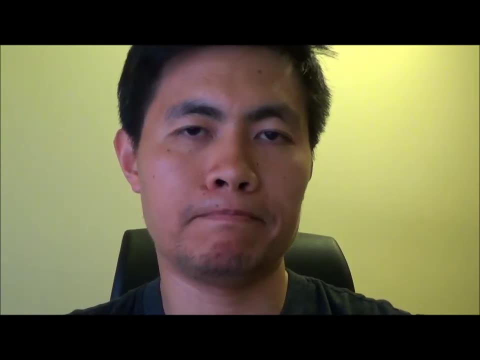 you two are stuck together. Now, when we expand that to the whole solar system, the planets revolve around the sun. The sun exerts the greatest amount of gravity of any object within our solar system. but why don't the planets and everything else fall into the sun? Because essentially, it's a balancing act between the gravitational pull of the sun, and gravity itself, and the centripetal force of those planets spinning around it. The closer the planet to the Sun, the faster it must rotate around it so as to not get sucked in. 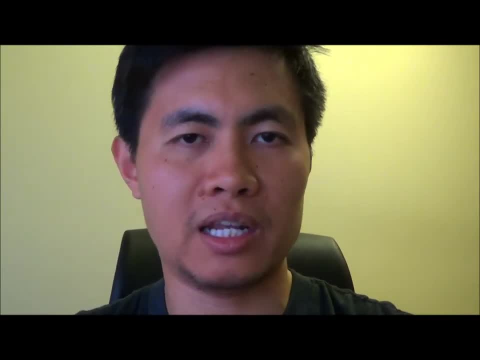 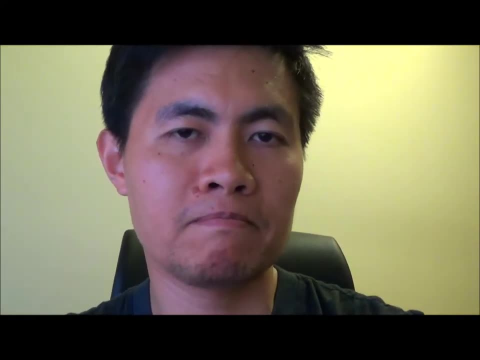 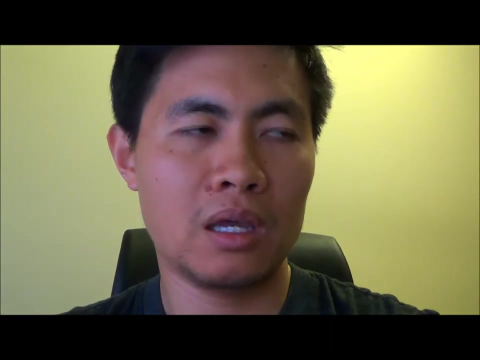 So, therefore, a Mercurian year is only 88 days, whereas a Neptunian year is about 165 years. Now, this concept is still very simple, But then let's move slightly away from that and look at galaxies. Galaxies are just like our solar system, only on a grander scale. 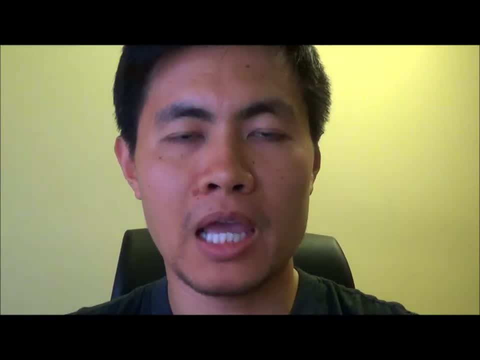 So when you look at spiral galaxies such as the Milky Way, you have a supermassive black hole in the middle which is the centre of all gravity within that galactic system And that supermassive black hole exerts all the gravity and pulls all the stars towards it. And it is the stars' spinning motion around the black hole that prevents them from falling in. So if you extrapolate the theory behind our solar system to a galactic system, the stars that are spinning closest to the black hole should be rotating at a much faster rate. 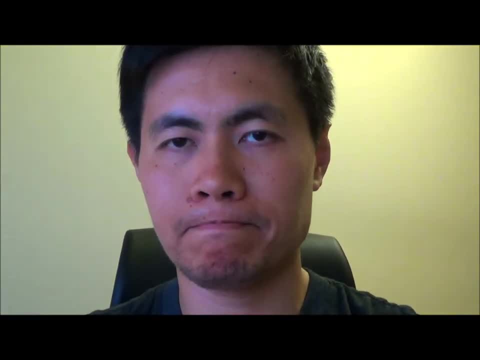 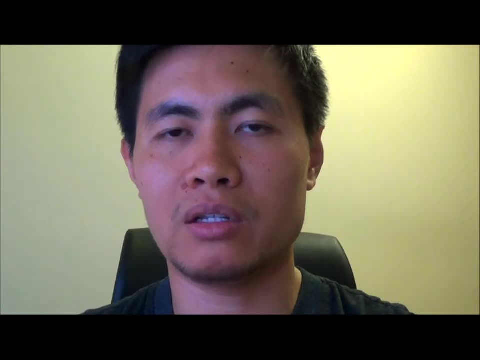 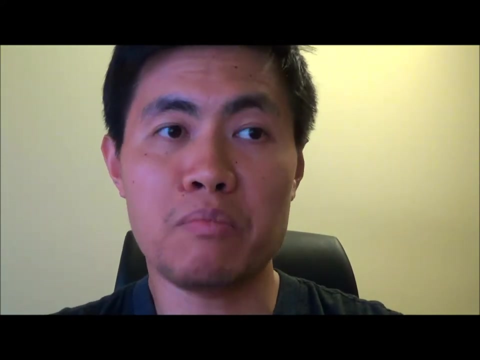 than those that are around the edges of the galaxy. Well, this is where cosmologists got stuck, Because when they look at the rotation rate of stars around the edges of the galaxy, they found that they are spinning at the same rate, if not quicker, than those around the centre. 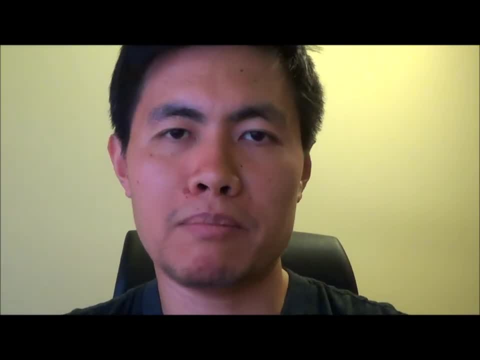 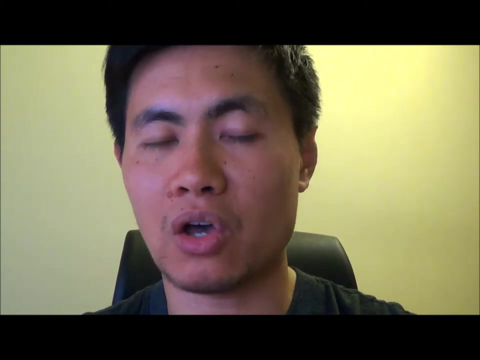 Which leads to a conundrum: There must be a lot more mass within the galaxy, and therefore within the universe, than we know about, because something is making those stars spin at the same rate on the radius on the outer edges of galaxies. 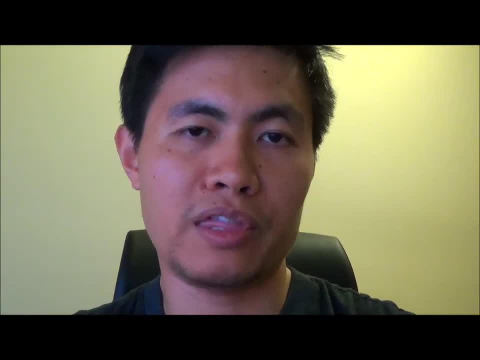 than the ones in the middle, And that led to the theory that if we look at the dark matter, we can see that there is a lot more mass in the universe than there is in the dark matter. And this is the difficult concept. 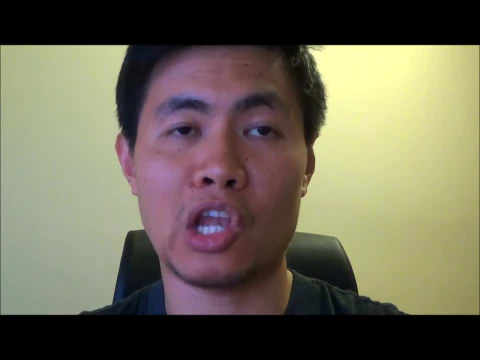 It turns out that more than 99% of all the mass in the universe is something called dark matter. You cannot see it because light just goes straight through it and you probably cannot touch it. It is supposed to be all around us. 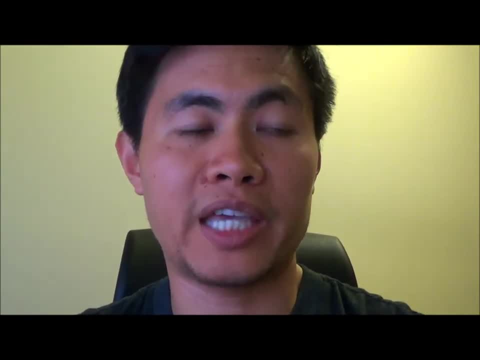 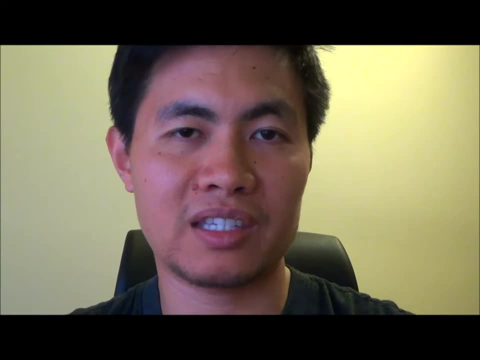 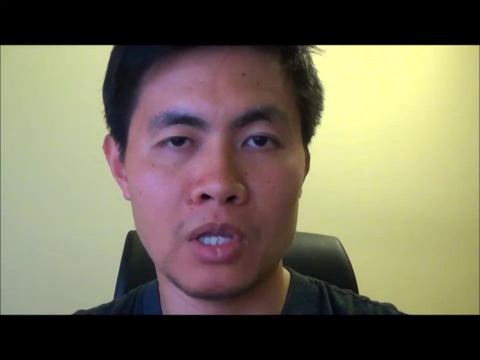 but, as I said, we can't feel it. And yet it comprises 99% of all the mass in the universe And I believe that the scientists that can essentially discover it and explain it will be deemed to be a worthy winner of the Nobel Prize. 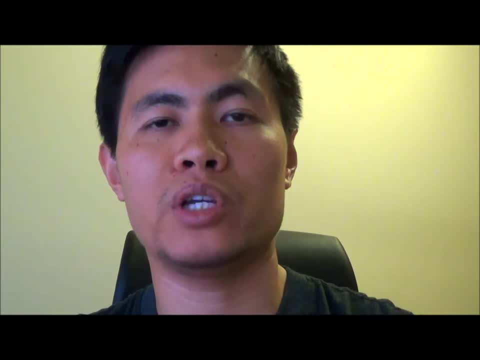 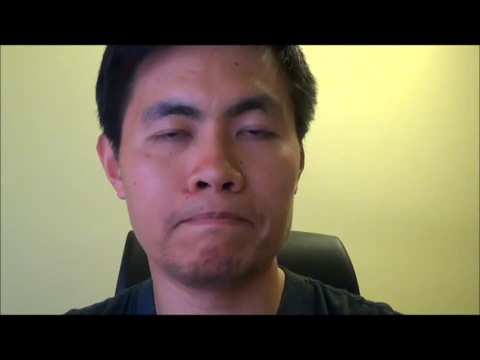 Not these idiotic Keynesian economists who just always push for stimulus. So dark matter is a very difficult concept. I'm sorry if that took a while. Dark matter is one of the most difficult concepts to explain and prove because essentially it's all theoretical. 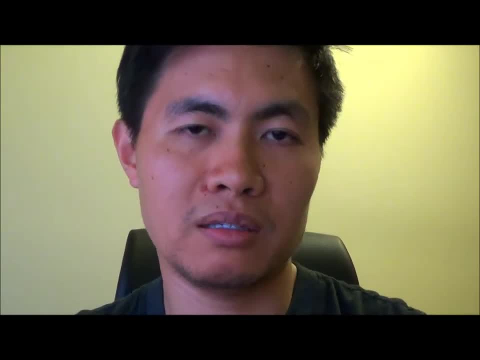 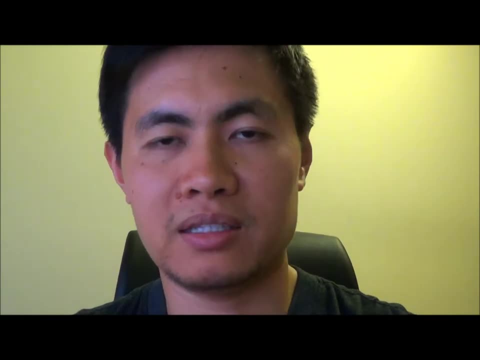 Now let's get back to financial systems and economic systems. There is essentially one law in economics that one has to look at to really look beneath the surface and understand how things work, And that is simply the law of supply and demand, And simply stated. if you have. if demand is unchanged and supply goes up, prices come down. If demand is unchanged and supply goes down, then prices, Sorry, hang on. If demand is unchanged and supply goes up, prices come down, sorry. If demand is unchanged. 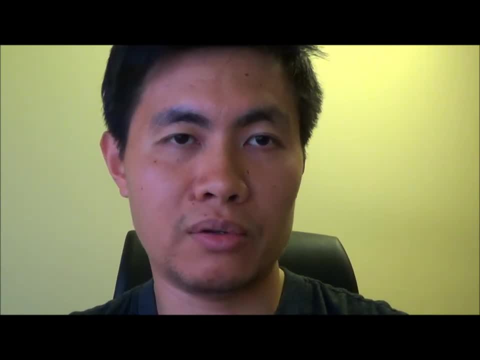 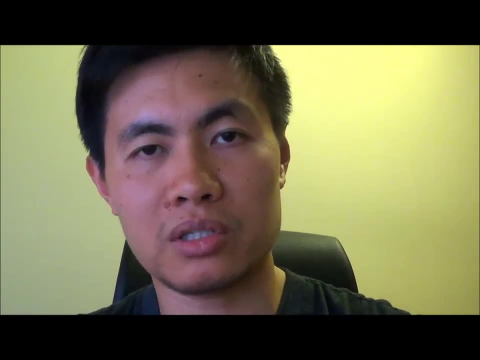 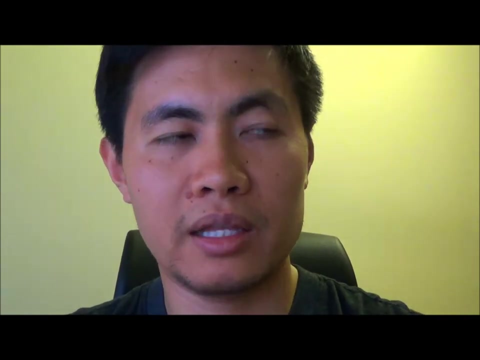 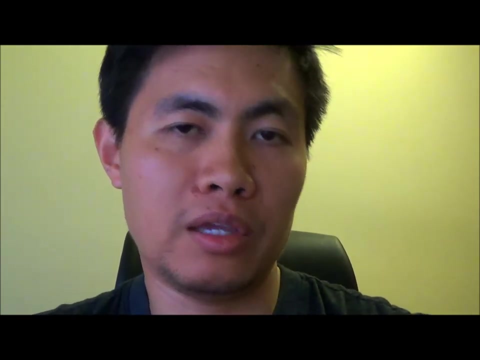 and supply goes down, prices actually go down Up. If demand goes up and supply is unchanged, then prices goes up, And if demand goes down and supply is unchanged, then prices come down. Very, very simple theory And it's a very, very simple concept to understand. 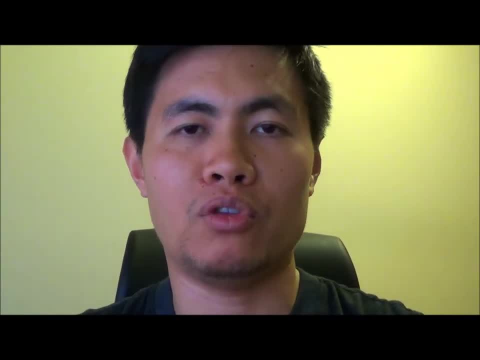 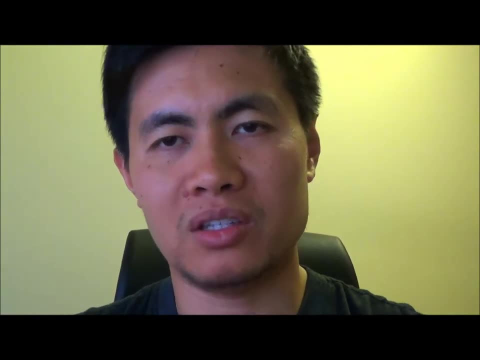 And everything revolves around it. whether it be the price of money or the price of goods and services, the price of anything that's out there is simply dictated by supply and demand. So even if you trade currencies or commodities or indices, everything comes down to the law of supply and demand. 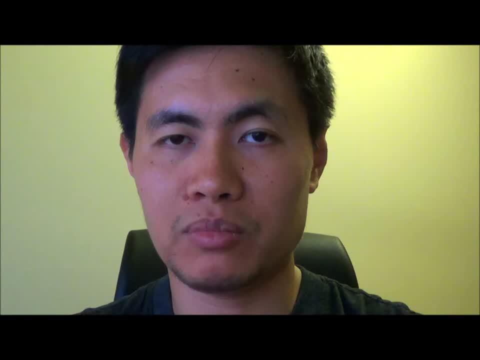 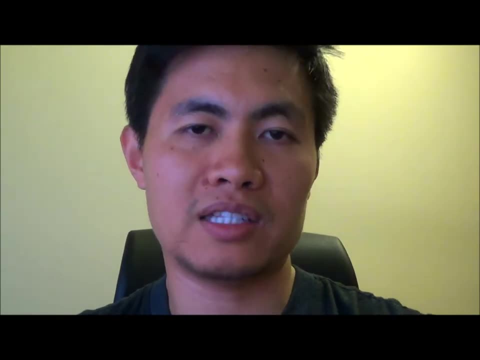 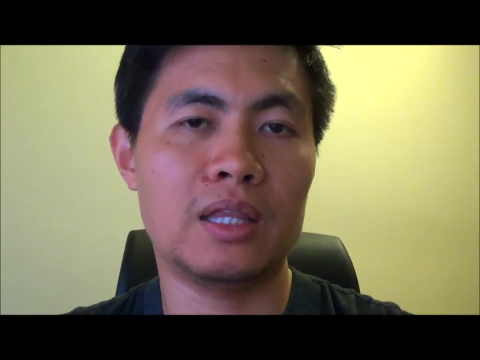 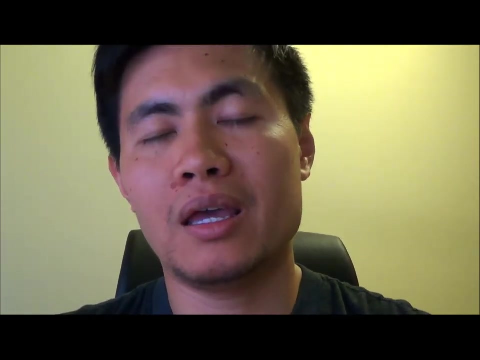 So, if you get your head around that concept, it's not too hard to understand the financial systems, if you can understand, as I said, the concept of supply and demand. But furthermore, one should understand the simple concepts of cause and effect. So if one does something, 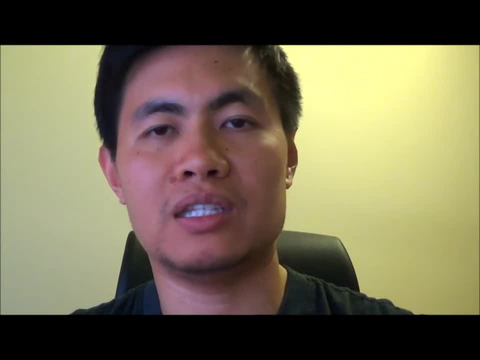 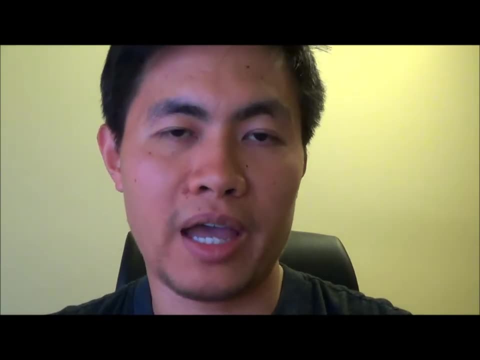 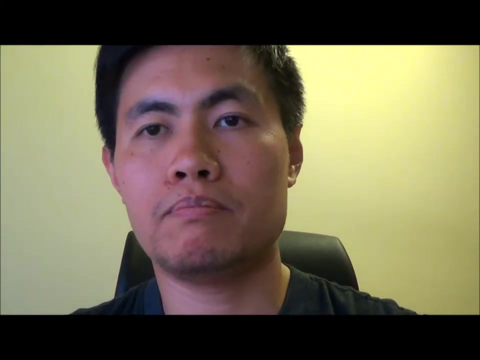 or one acts in one way, an effect is going to come as a result. So if you were to hit a nail with a hammer, the nail is going to get embedded into the timber or whatever surface that you're nailing it into If you push somebody. 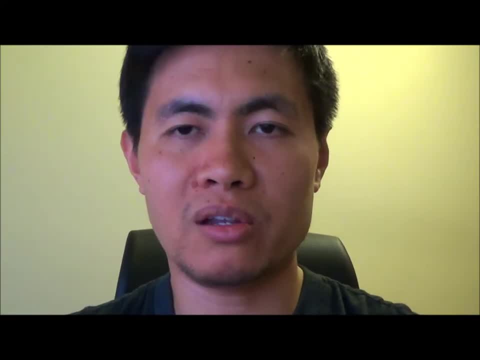 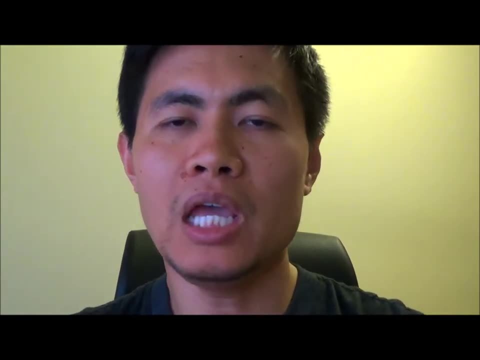 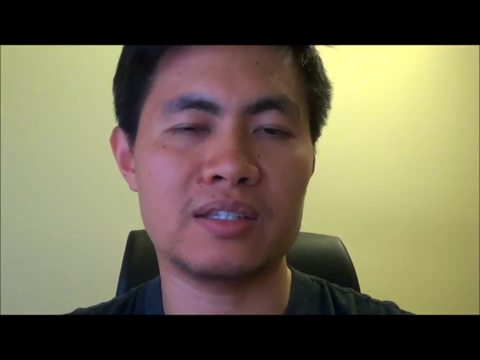 that person's going to fall down. So there's a lot of cause and effect And within financial systems it's the same thing. If central bankers decide to print a crapload of money and everything else stays the same. the cause: the printing of money. 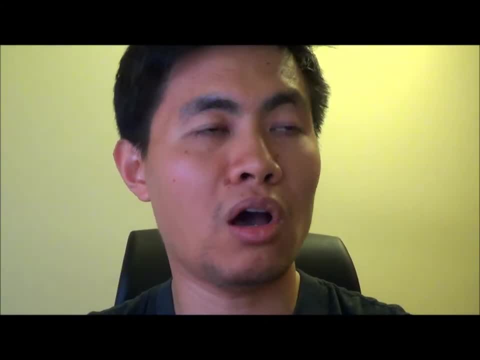 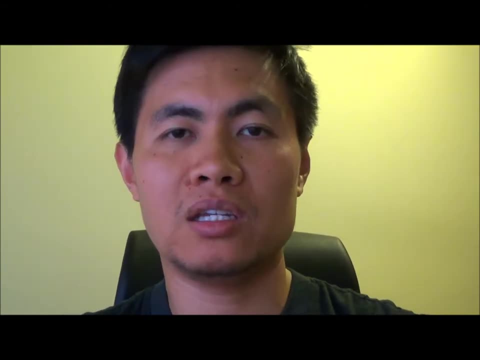 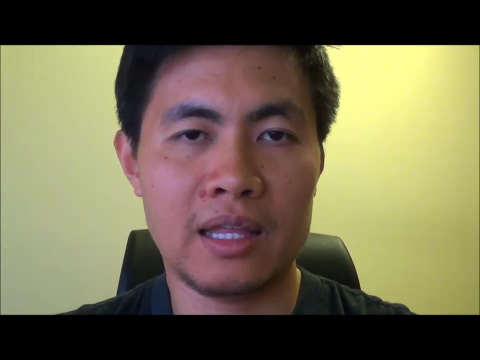 is going to lead to a devaluation of that money. in itself, That's a very simple concept to understand, But yet the economists and the central bankers and all those idiot lemmings, investors or traders out there who are trying to trade against the actual concept, may win out at first, because the central bankers may try and stifle the effects of the action that they've taken. But essentially the free market will catch up when other factors come into the equation and everything gets back into balance. So it doesn't matter how much. 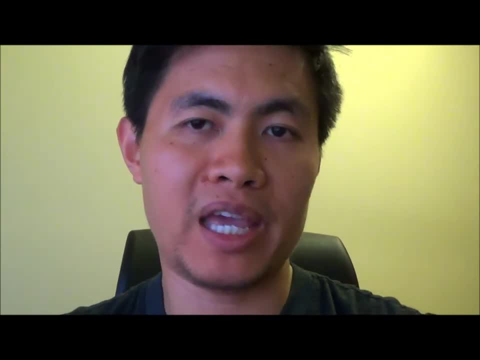 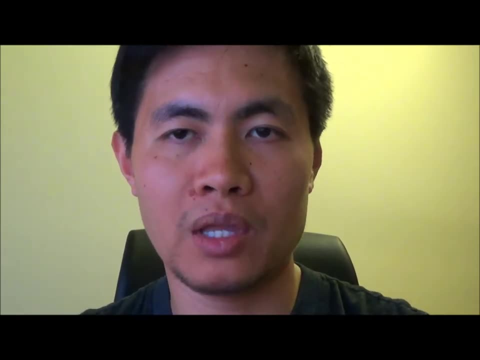 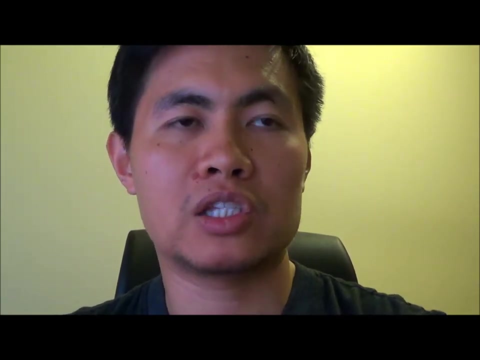 the Fed wants to lie about there being no inflation because, first things first, the definition of inflation is an expansion of the money supply. First myth: totally unfounded, So to say that there's no inflation, but yet you've quadrupled the money supply. 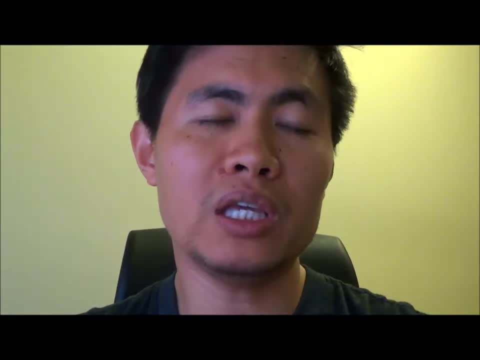 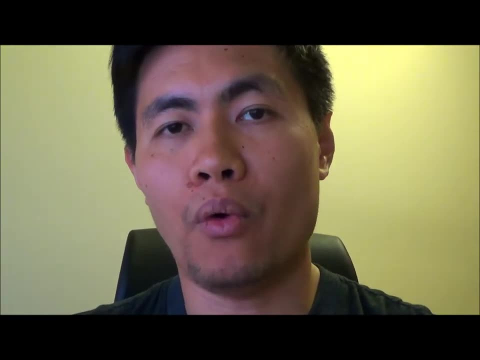 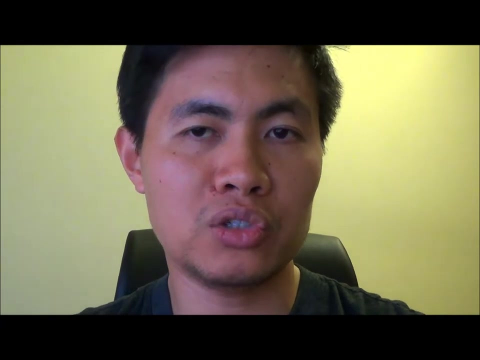 is an absolute lie in itself. Now, if we take a more layman's view of what inflation is, and that being interpreted as the rise in prices of goods and services, well, through the use of statistical manipulation and selective withdrawals of items that have gone up too much, the Fed and other government officers can lie about the rate of inflation. But essentially, if you print money and that money is now in such great supply, chasing a finite amount of goods and services, then you know that there must be rise in prices of those goods and services. 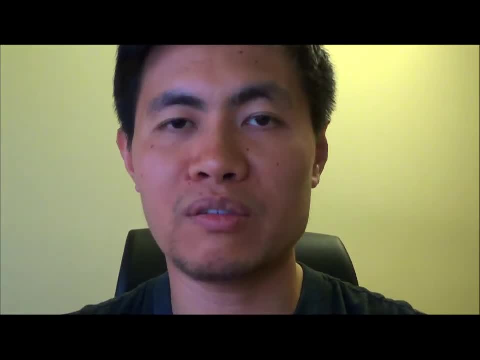 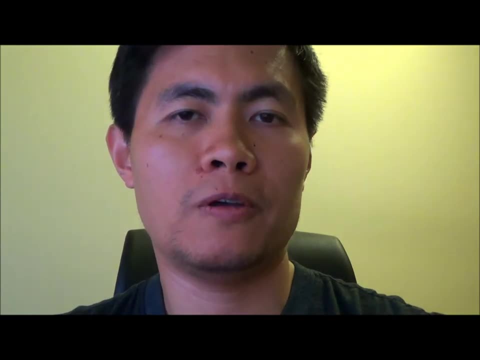 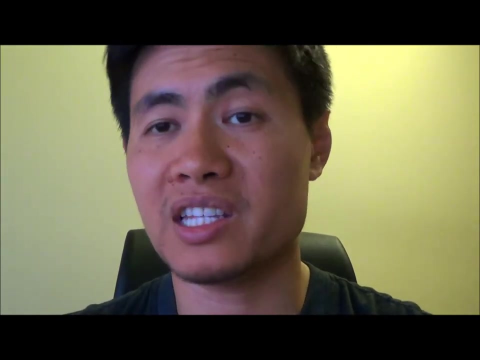 because you've got so much more dollars chasing all those finite amount of goods and services. It's a mouthful. So whenever you hear about the lack of inflation or even scarily deflation, which is actually what the free market wants, but unfortunately, because of the amount of debt that the US and other large Western democratic countries have lain themselves with over the past decade or two decades, especially the US in the past five years. there is nothing else that they can say except that they need more inflation and that deflation is going to lead. to a destruction of the financial system. They have to say this because, as the debt gets bigger and bigger, the only way to get rid of it is to have an inflationary default, in that if you print enough money to make that money meaningless, the numbers become meaningless. 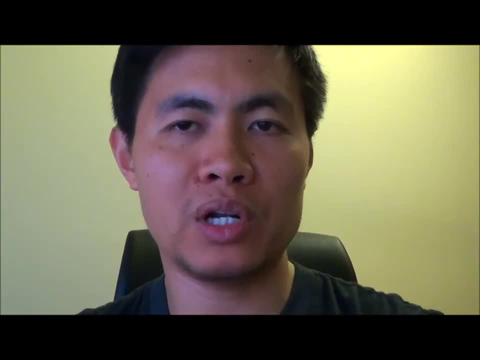 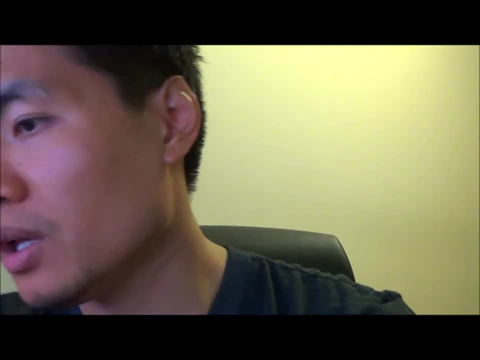 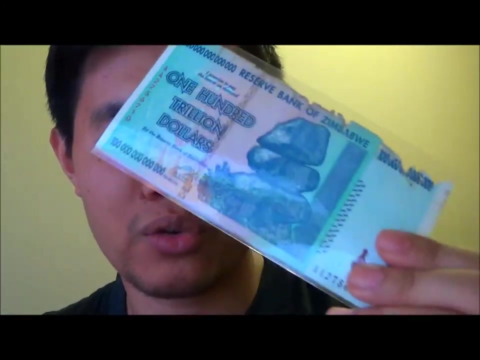 within the currency, then all that debt, that $17 trillion as it stands today, will become meaningless. And if you don't believe that something like that can happen, I've always loved this. but the Zimbabwe currency- $100 trillion- That's the extent that you can print money. 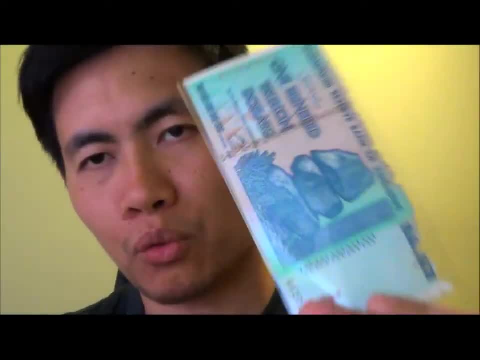 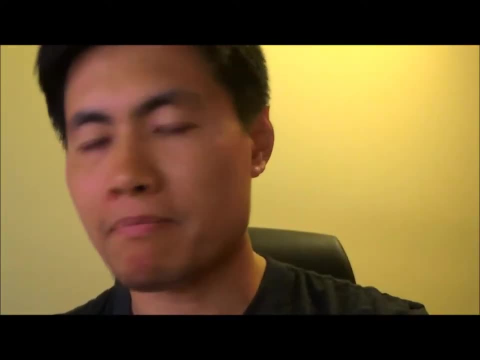 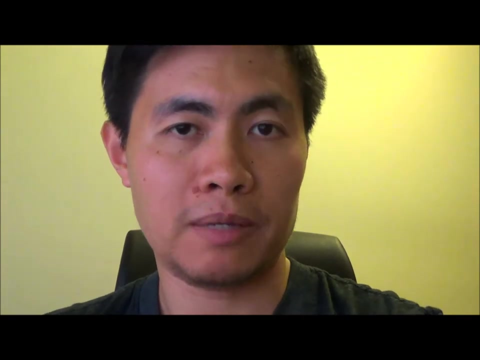 until it has no more meaning. That's one followed by 14 zeros, And yet this note could not even buy you a square of used toilet paper. It essentially is not currency anymore, and nor does it deserve to be, But America is fast heading down that track. 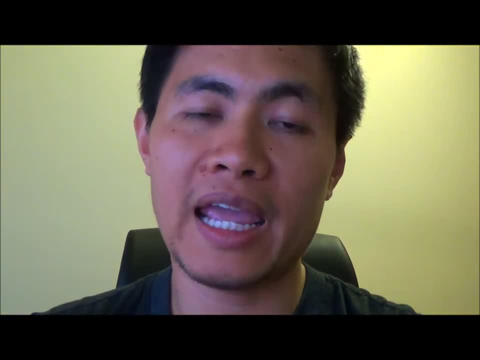 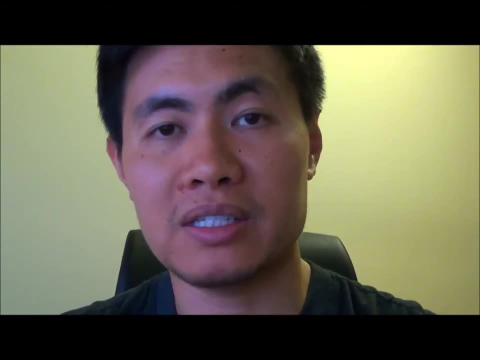 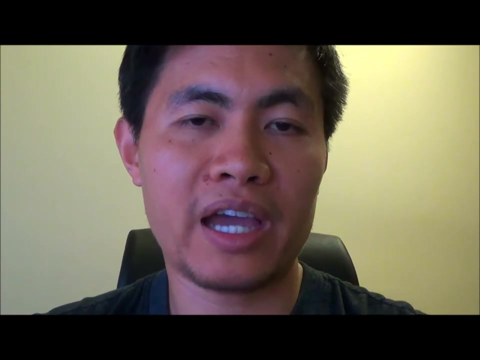 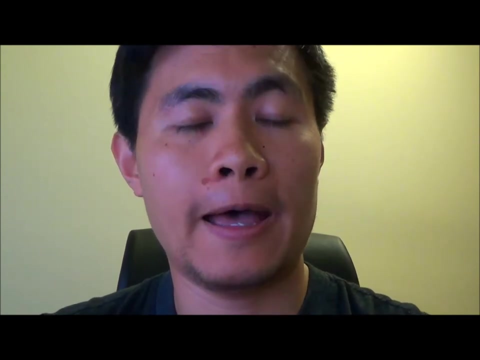 and it's not without any sort of discretion that the Fed and policymakers are saying that they're actually not doing that And in fact you can see a lot of actions, especially coming up in the following discussions over the Fed and the policymakers, that they try. 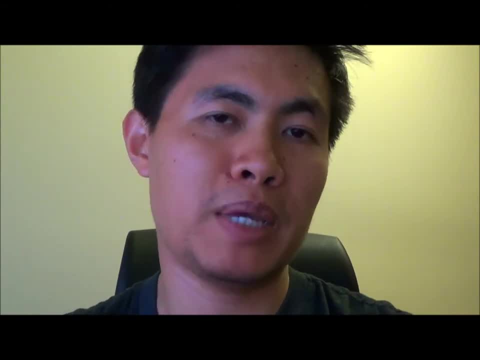 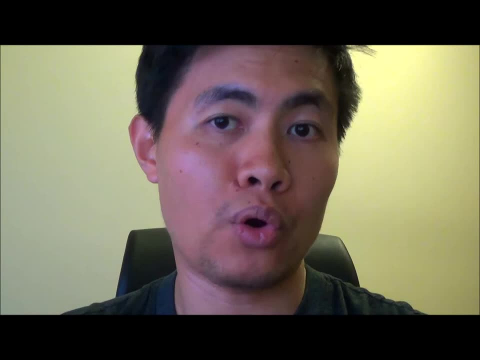 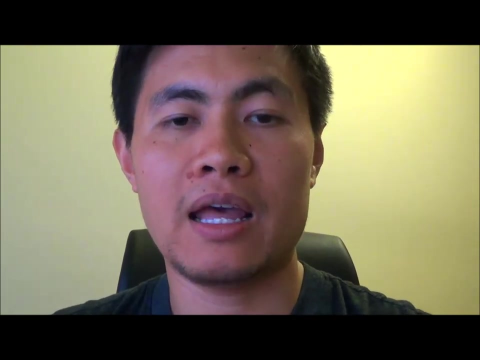 they put a positive spin on their actions and, in fact, they artificially create situations where the rest of the world believe that they're doing the right thing. and yet everything continues unabated And the total elimination of their debt through inflation is high on their cards. 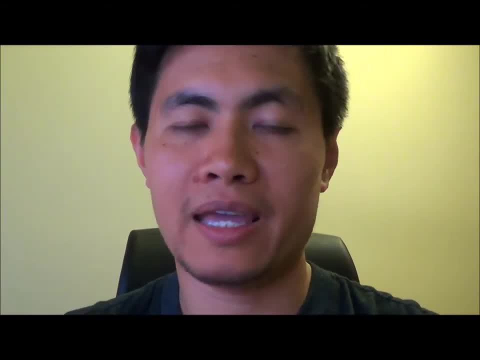 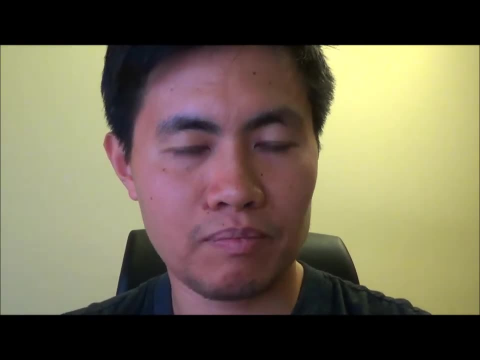 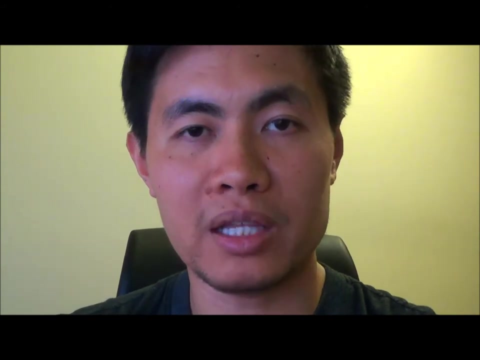 But essentially nothing will change And it doesn't matter if the Fed tries to artificially manipulate the markets, whether it be the bond market or the stock market or the housing market, through the manipulation of interest rates, both through lowering the Fed's funds rate. 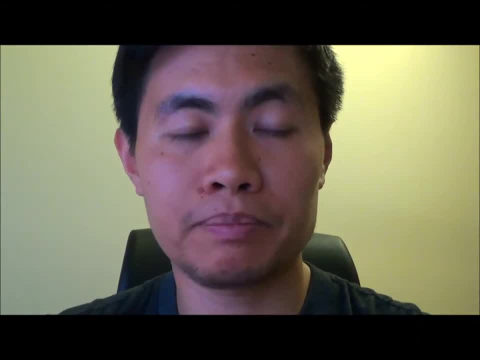 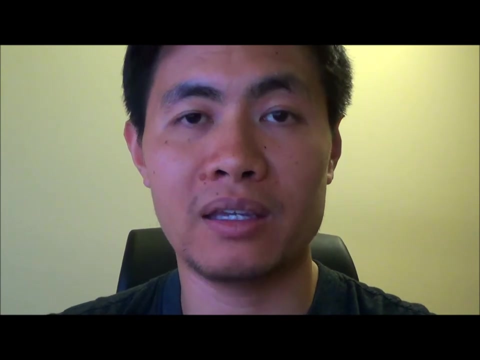 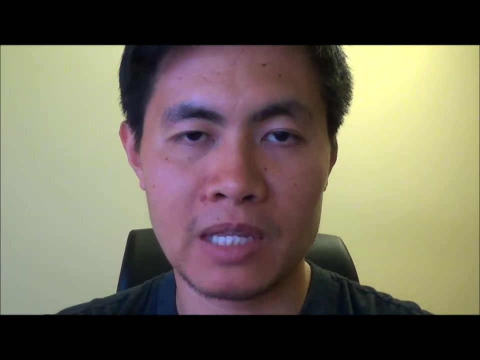 down to almost zero and through asset purchases, of both mortgage-backed assets and their own treasuries, just to keep rates low. But essentially that's the two tools that the Federal Reserve has in its tool bag to try and help revive these zombie economies of theirs. 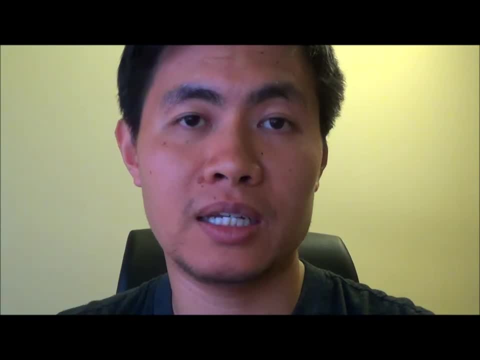 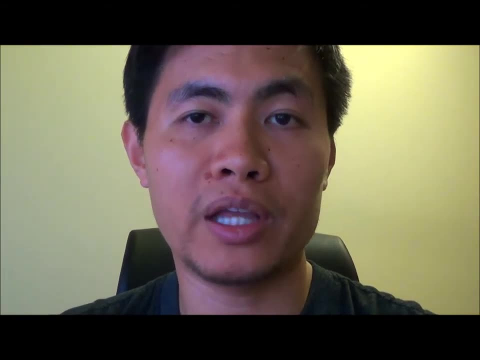 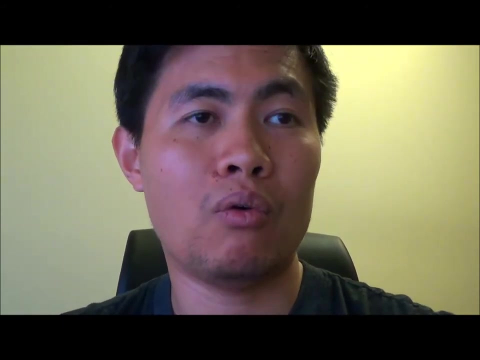 So even when you look at supply and demand, interest rates are simply the rate of supply and demand of money. So a very, very simple concept of interest rates is that when there is a high demand for money through the banks or through loans, 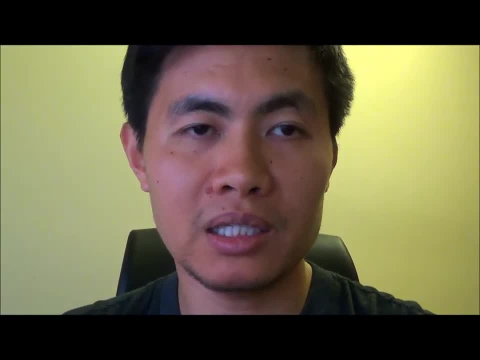 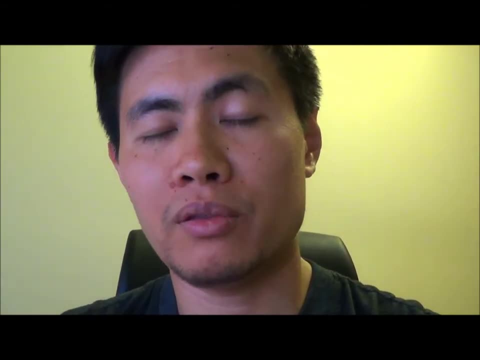 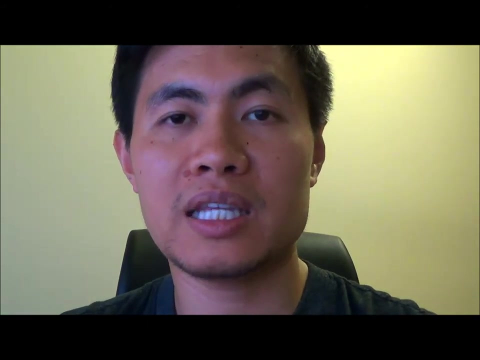 interest rates have to go up. When there is lower demand, then interest rates just come down. A very, very simple concept. And by the Fed artificially clamping down on interest rates it sends out false signals to the economy that while there is low demand for money, 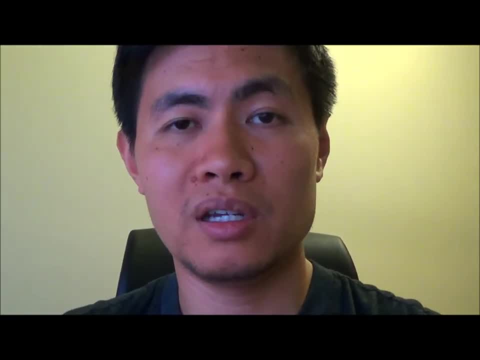 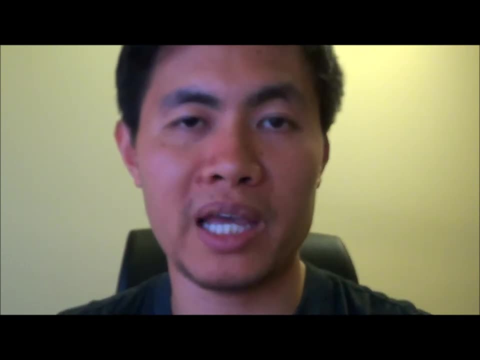 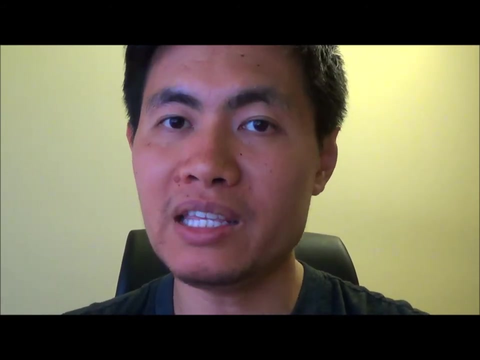 so therefore, you should borrow as much as you can and take advantage of it, But essentially, the consumer is tapped out and companies are issuing debt at a record pace to take advantage of these unbelievable interest rates And suckers who believe that the economy is recovering. 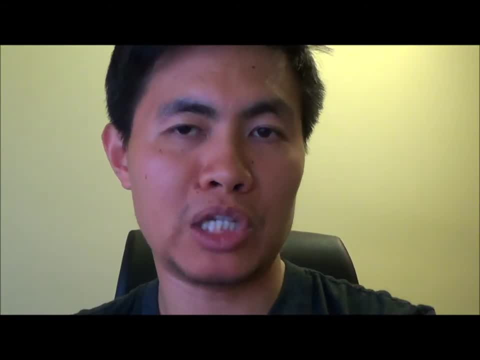 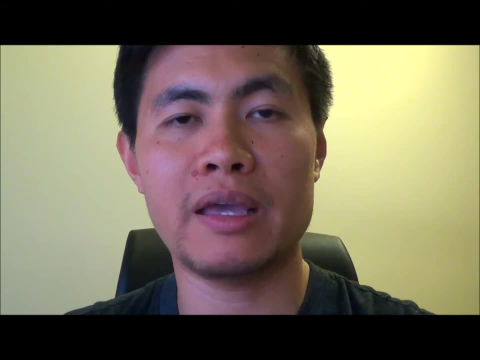 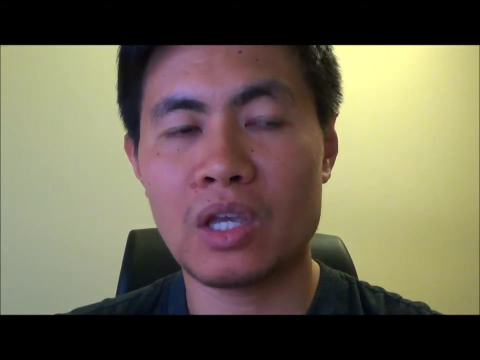 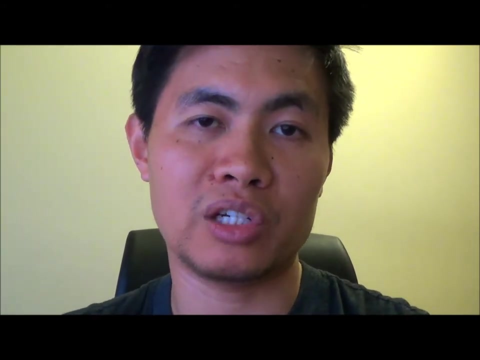 and yet interest rates are so low, are in for a big shock when the free market returns and the Fed is totally unable to do anything about the consequences of that happening. So essentially you can clamp down on bond yields by purchasing assets, But that's on a diminishing return. Because as your balance sheet grows and as the amount of debt grows, you have to purchase more and more and more bonds just to keep the rates at the same pace, Because the free market and inflation dictates that rates must go higher when you have so much demand for money. 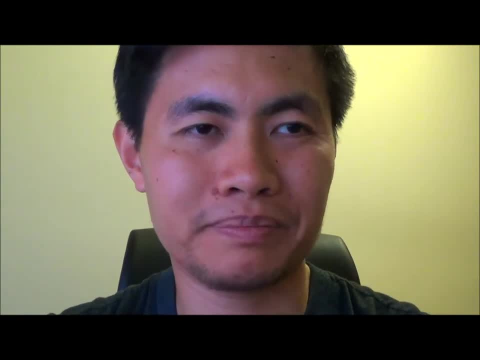 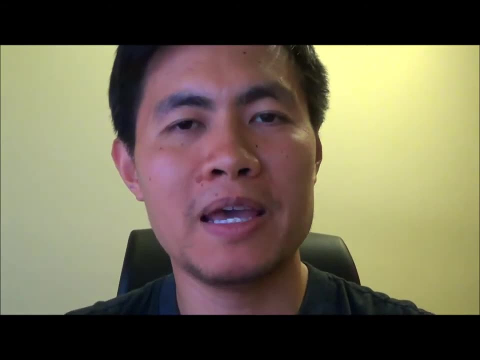 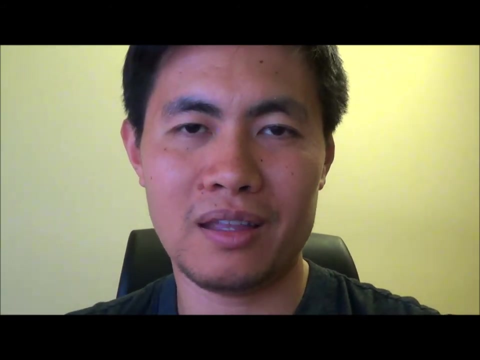 And so, as a consequence, I believe that the Fed, I believe that the Fed will never taper- This is the subject of the next video- But it cannot taper for the simple reason of its own destruction, the destruction of its own balance sheet and the structural default. 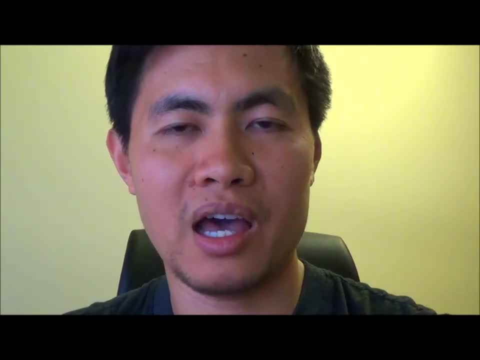 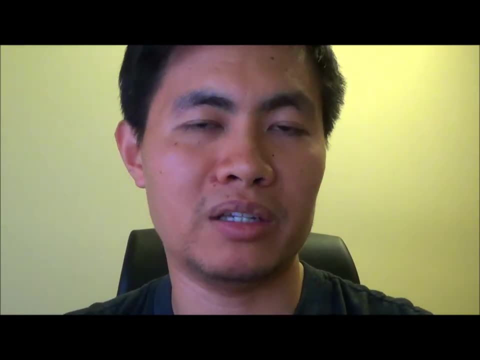 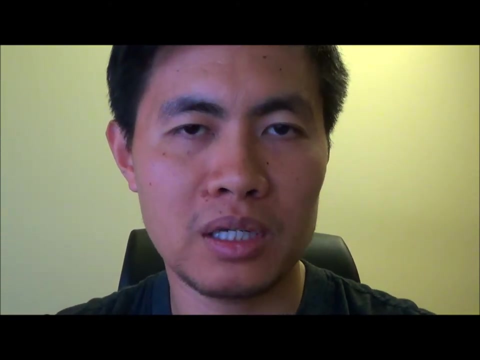 of the American government. as a consequence of them, tapering, And I mean a proper taper, not some bull dust, $5 or $10 billion taper. So keep on reading, Keep on getting informed And don't get overwhelmed when you listen to financial commentators. 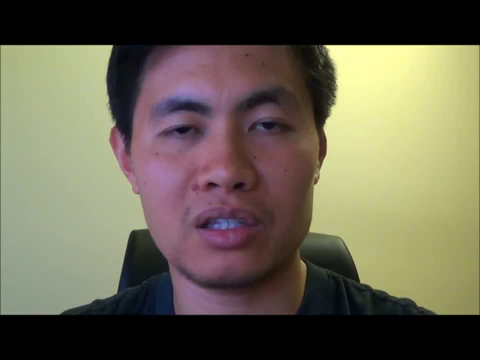 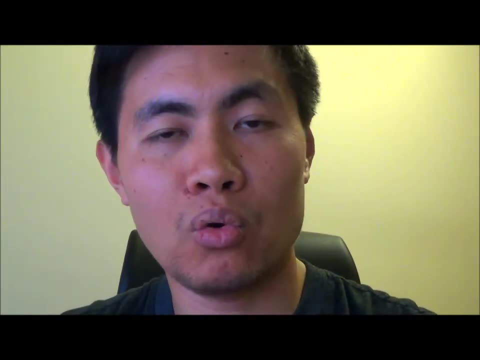 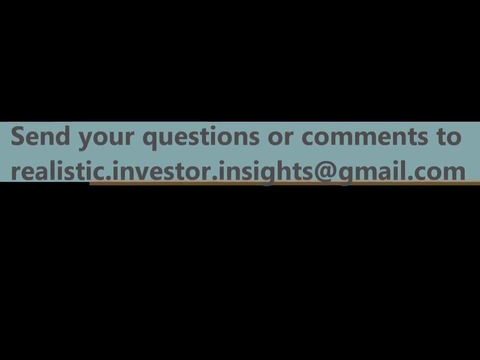 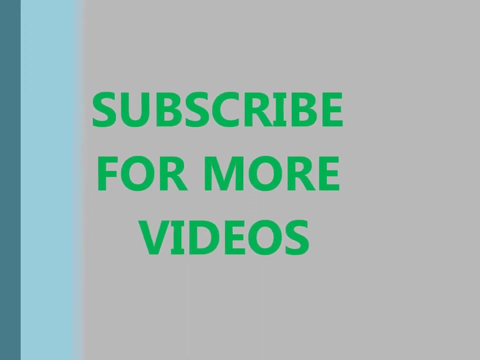 economists or just idiots who want to sound really intelligent through the use of big words. But essentially all the concepts are very simple. There is a lot to be told in a short time And I am also not going to get into all the details of financial account. but will give you some examples, or some examples of how this works. But I will share some things that I believe will give you a little bit more insight to how you should handle your financial statements. Let me talk about a very common and very common example. of how you should look at it. There is a term called the financial accounts system.